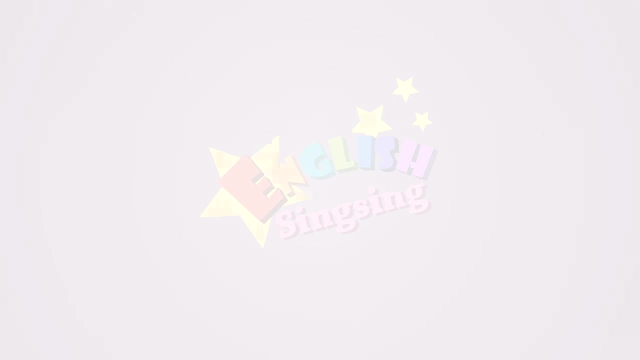 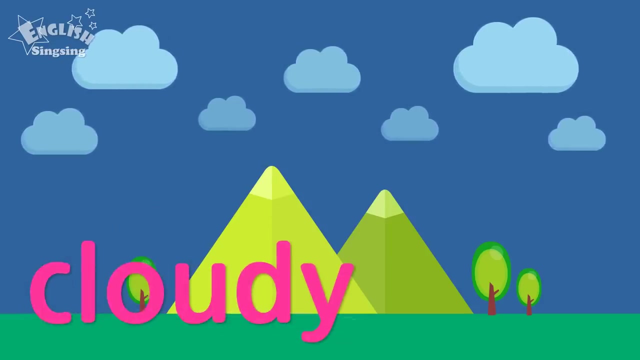 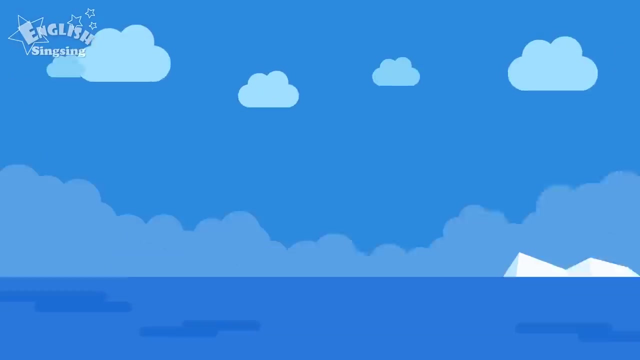 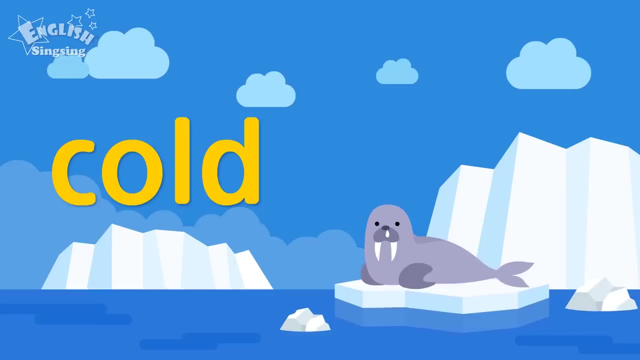 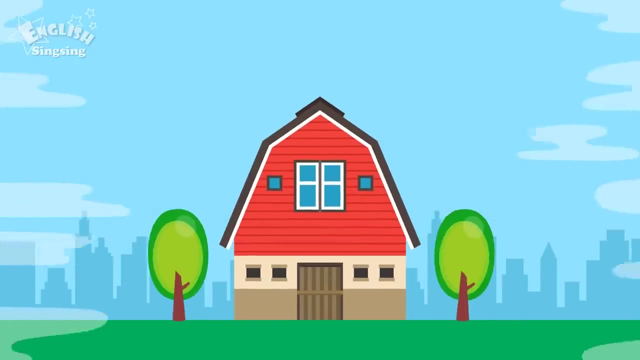 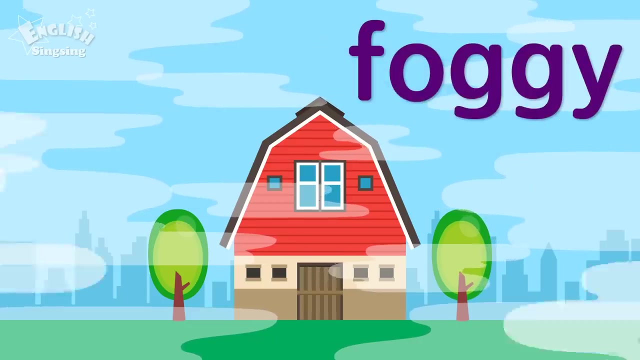 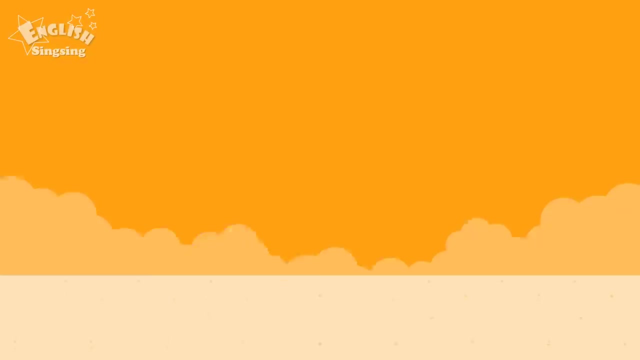 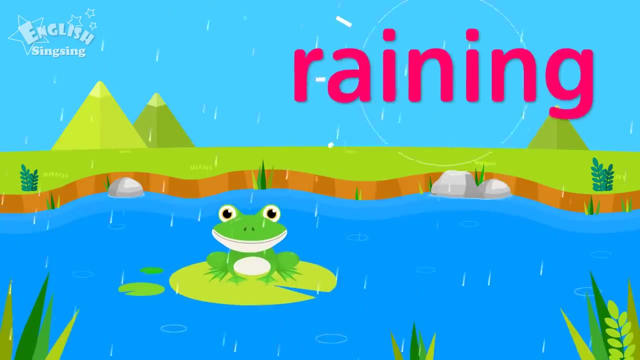 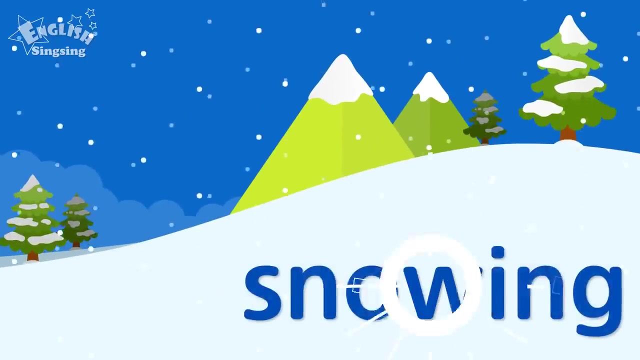 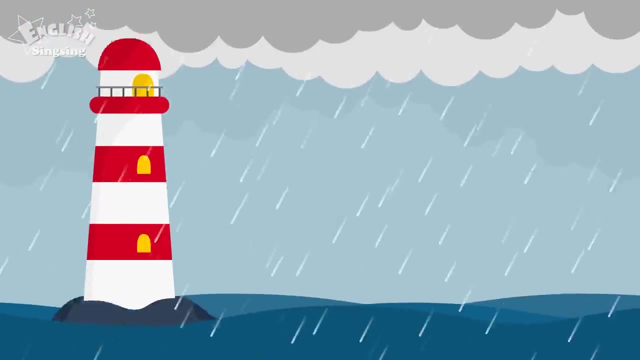 English sing-sing: weather: cloudy It's cloudy, cold, cold It's cold, foggy, foggy It's foggy, hot, hot It's hot. raining, raining It's raining, snowing, snowing It's snowing. stormy, stormy, stormy. 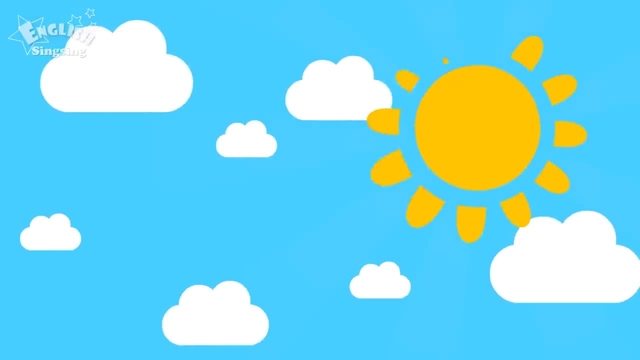 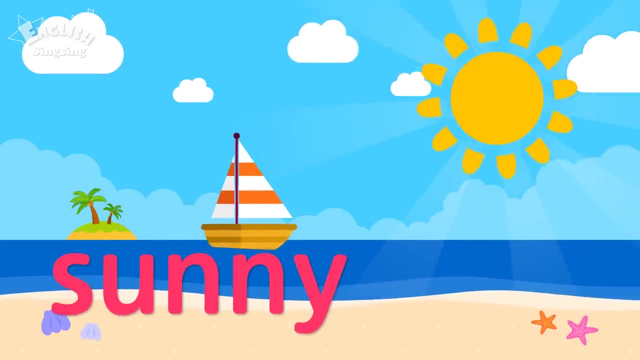 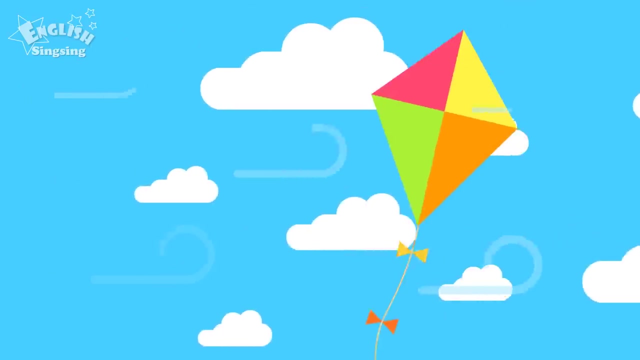 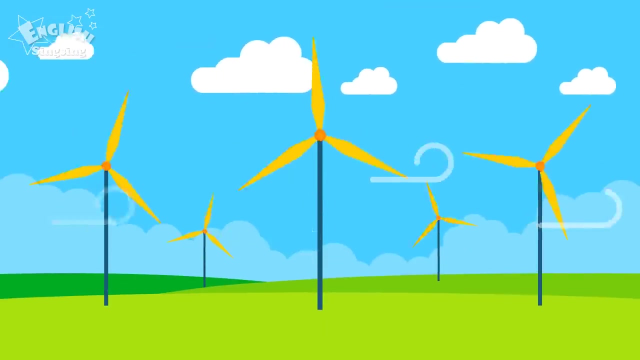 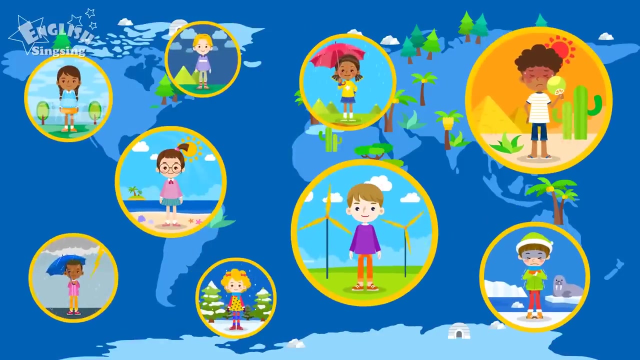 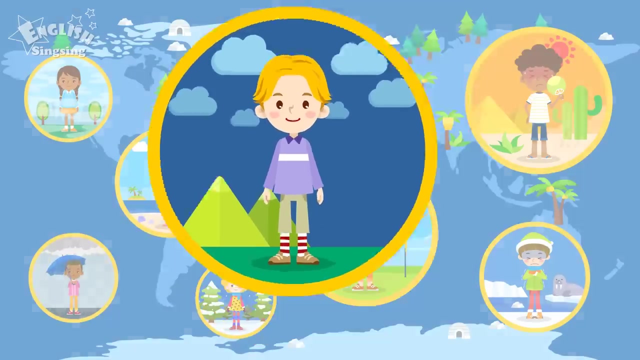 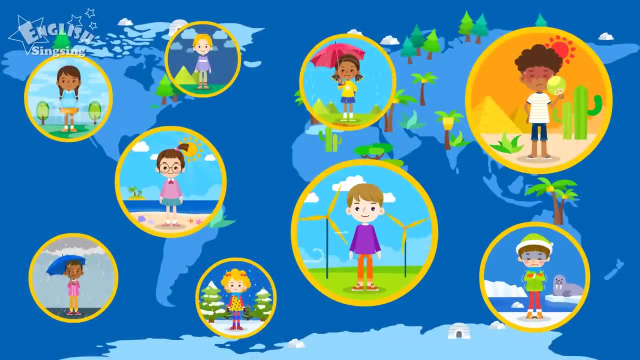 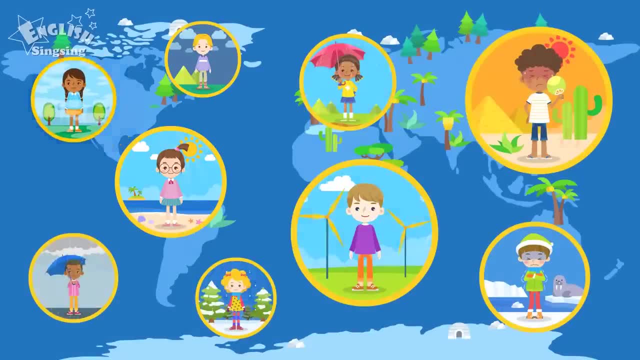 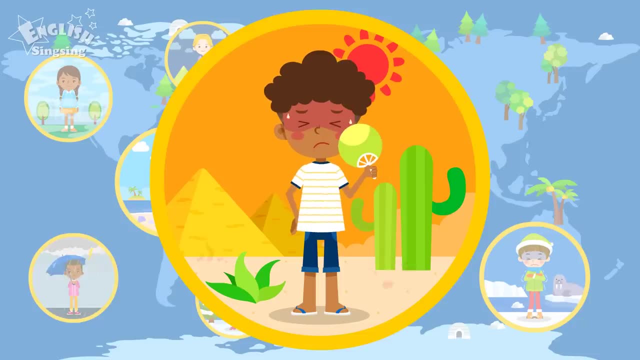 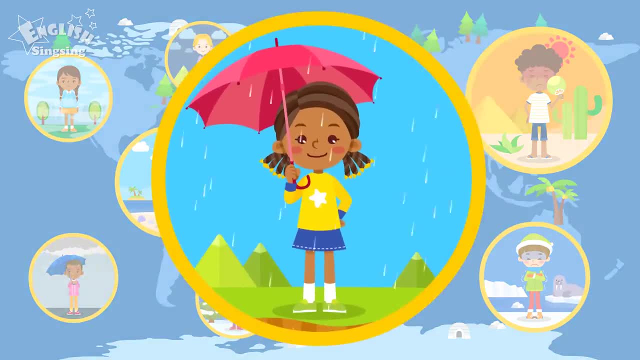 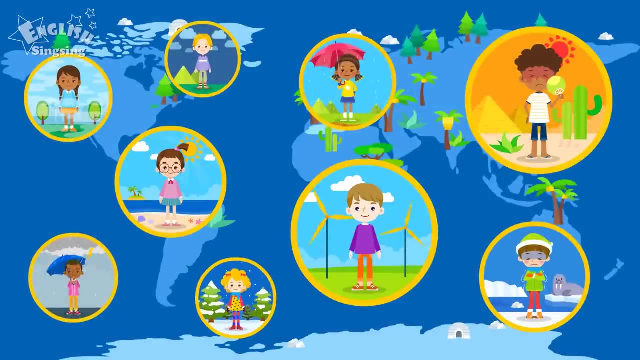